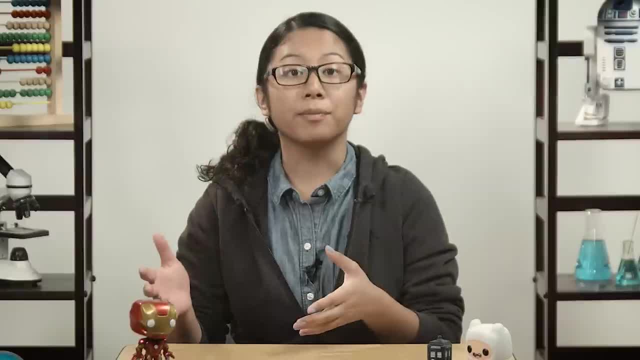 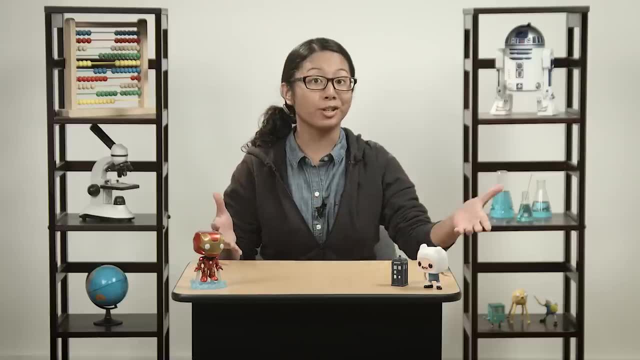 is anything made by combining two or more different things, And some kinds of mixtures, like the fruit salad we had at our picnic, can be separated back into the substances that made them, But that's not true about all mixtures, Sometimes mixing things together. 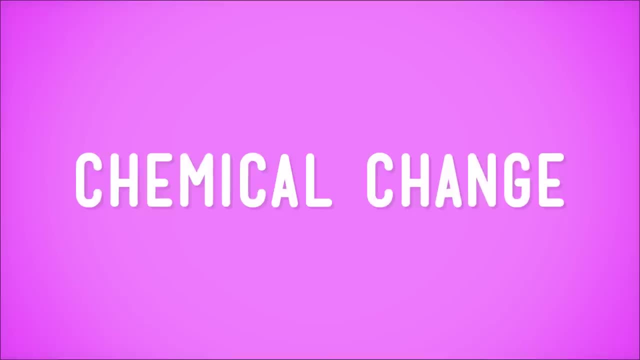 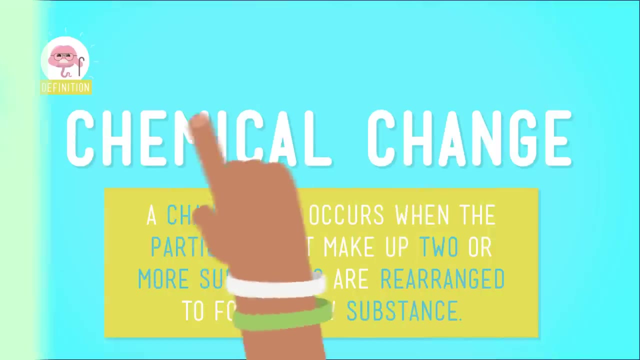 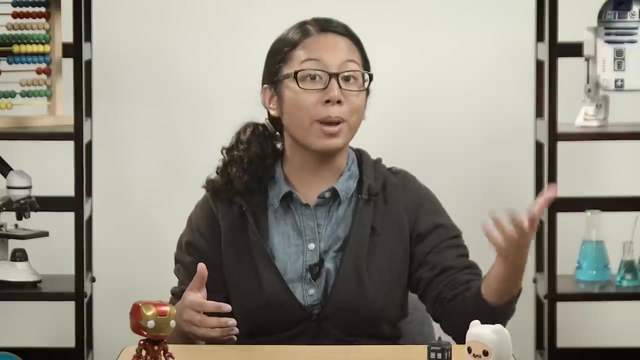 makes a whole new substance. We call this a chemical change. But what is a chemical change? A chemical change is a change that occurs when the particles that make up two or more substances are rearranged to form a new substance, Unlike the mixtures from our picnic chemical. 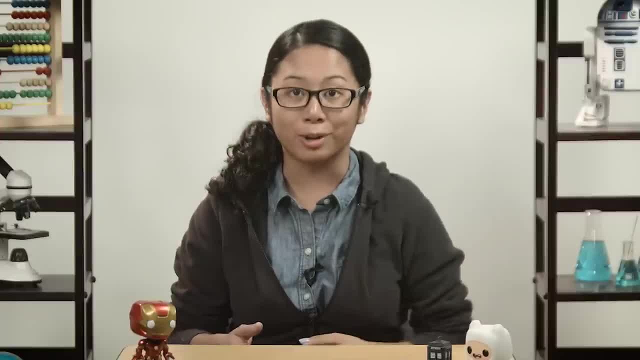 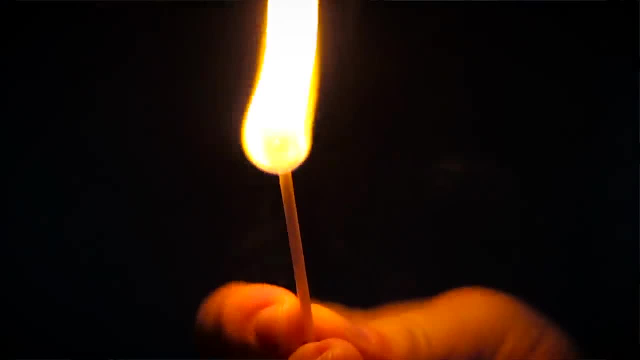 changes usually can't be undone. Let's observe an example of a chemical change. Observe people, We're not trying this at home. When we observe a lit match, we see that the match burns. As it burns, it changes into: 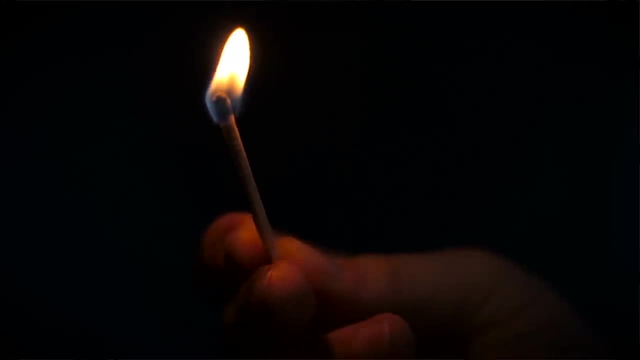 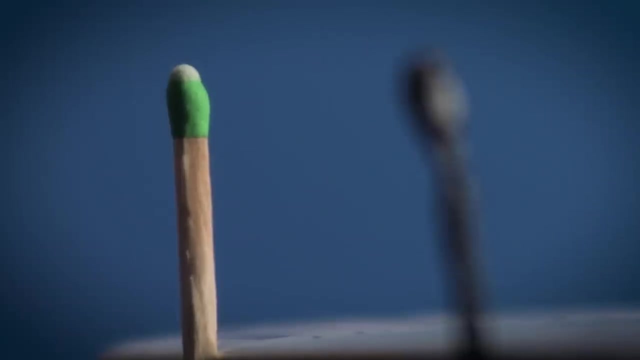 burned wood and ash. We can't change this ash back into a match, so burning is an example of a chemical change that can't be undone. But wait, There's more. Chemical changes often make matter, change color, like the blackened remains of the match. 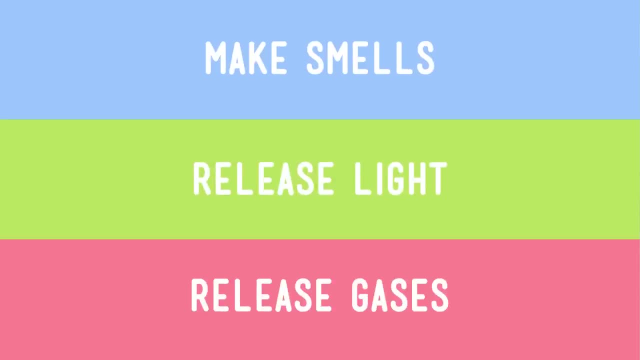 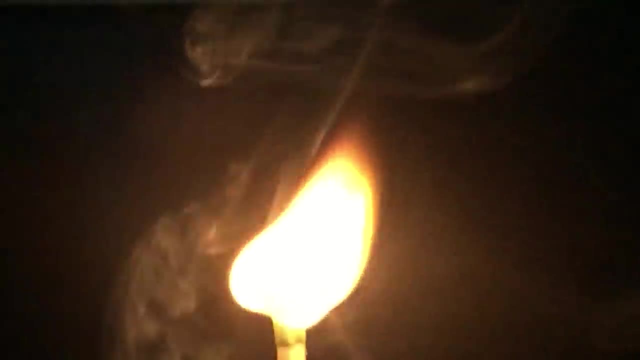 Sometimes chemical changes make smells or release light or gases, and lots of chemical changes require either the giving off or taking in of heat. A burning match gives off light, smoke and heat. All of these things are evidence that when we look at a burning match, we're 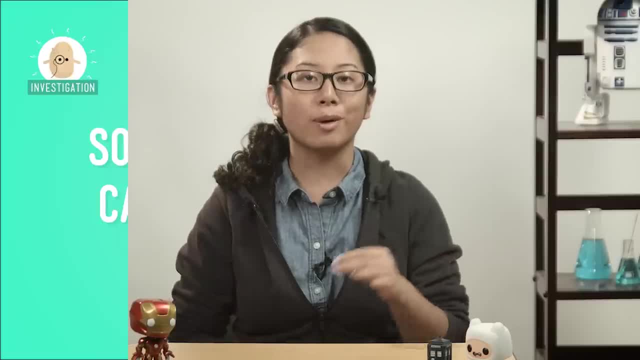 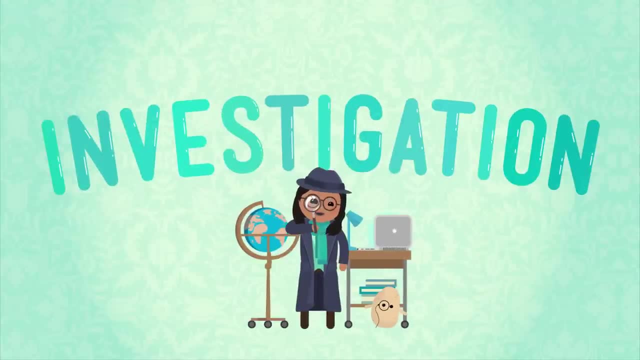 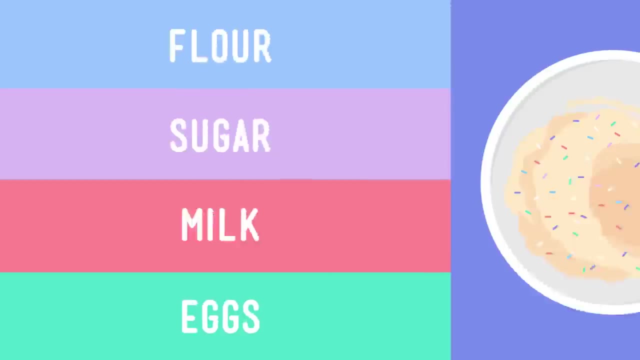 looking at a chemical change. Now we can do a simple investigation to show how some chemical changes can yield a seriously yummy result. When we mix the ingredients of a cake, we're mixing together different kinds of matter. Say, you have flour, sugar, milk and eggs. When you put them in a bowl and stir, you're. 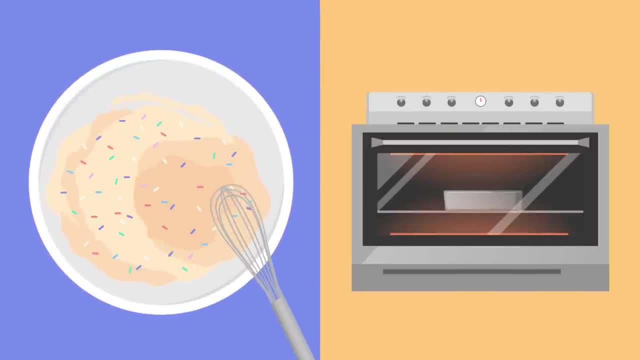 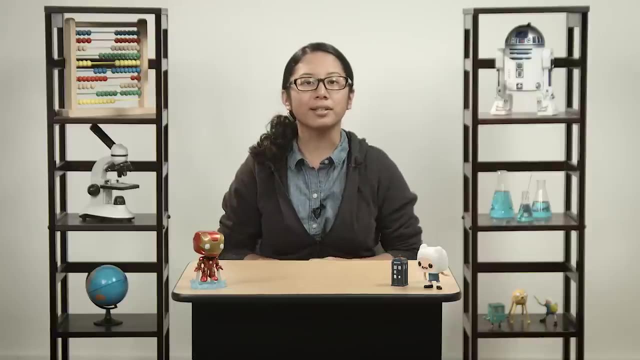 mixing several different substances together to make cake batter, And when you pop this mixture into the oven after a short time, you have a new substance Cake. Now, before you eat it, let's check this science cake for evidence of a chemical change. 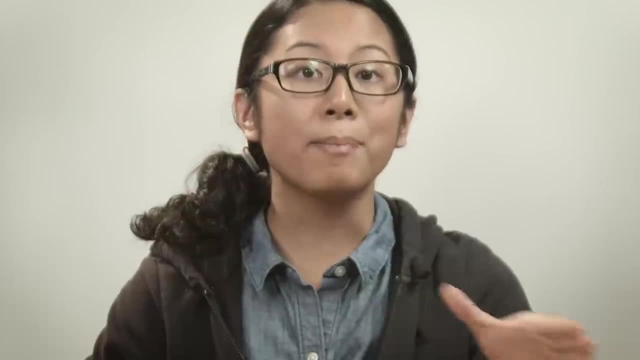 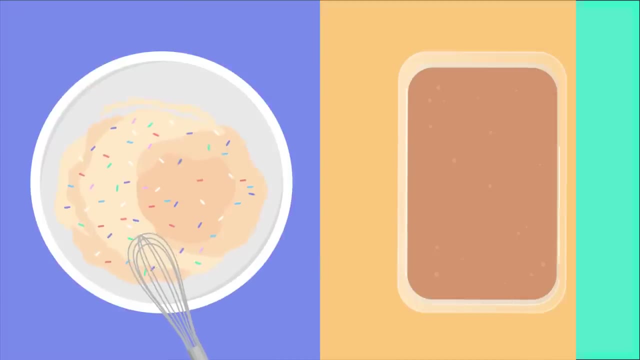 Did the reaction give off or take heat? Definitely The cake batter needed the heat from the oven to change into cake. If we left the batter on the counter, it would stay batter. If we left the batter on the counter, it would stay batter. Is there a color change? Check. 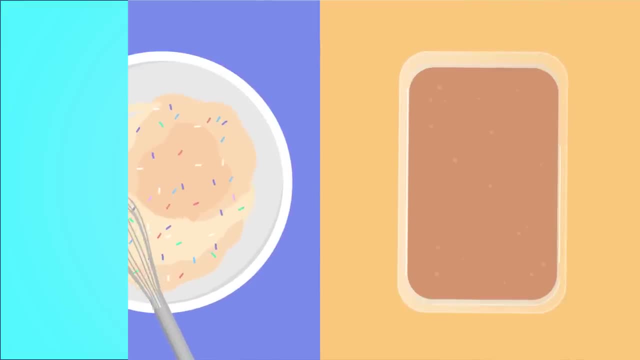 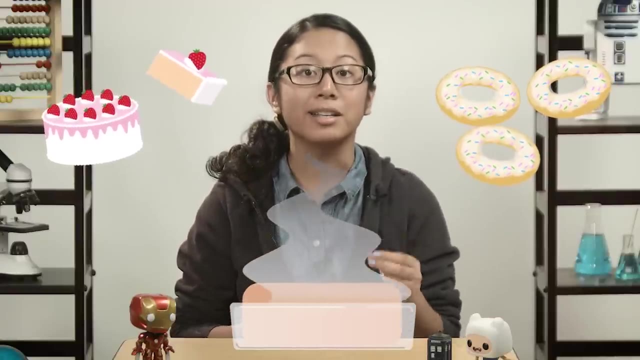 The batter in the pan was yellow and now it's a nice golden brown. Is there any smell? Well, if you've never been in a bakery or some grandma's kitchen or just never smelled a cake baking, then I feel bad for you, because it smells amazing. Were any gases released?